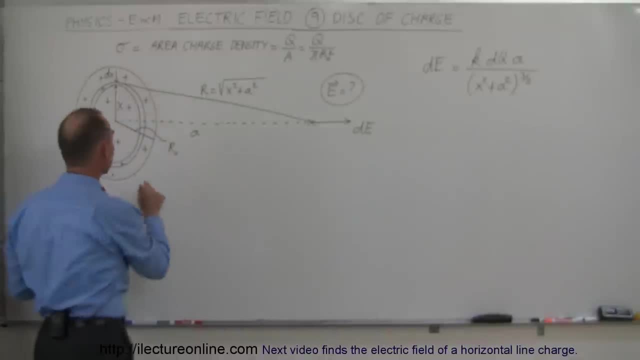 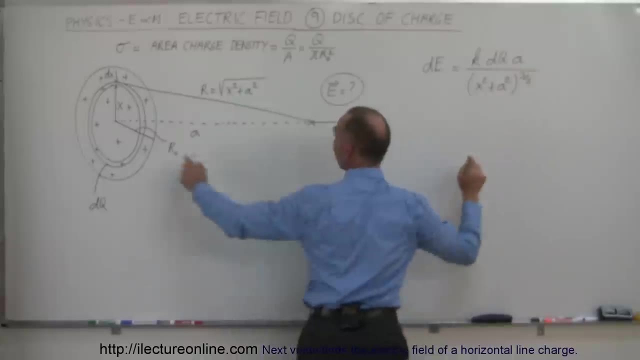 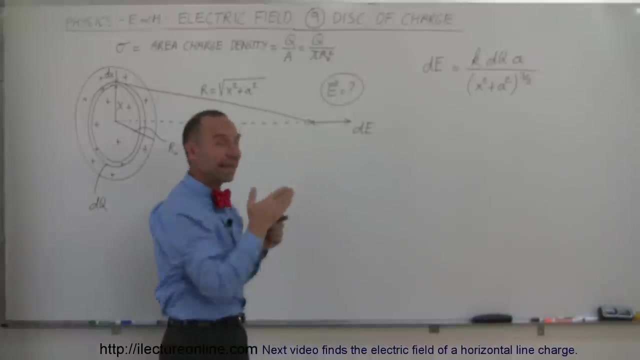 field caused by the full disk, but the equation for the charge caused by the little ringlet from last video was equal to K times the charge, DQ times the distance to the location from the disk divided by x squared plus a squared to the 3 halves power. though the difference between this and the answer of the 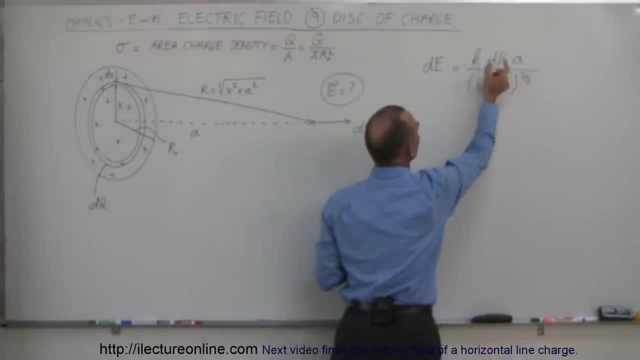 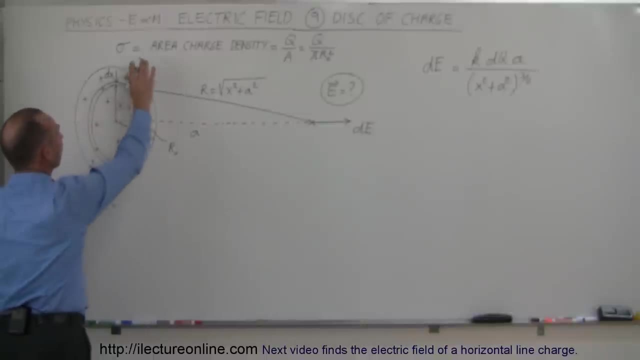 previous video is that we now just only have a small amount of DQ instead of the total charge on the ring. now the DQ here. how do we find that? well, the DQ is equal to the area charge density times the area of the little ringlet which we'll 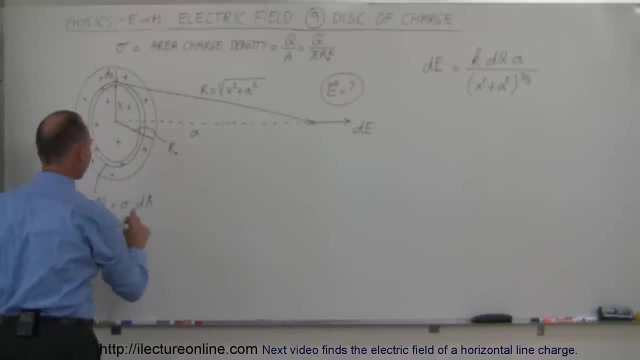 call DA, and so this is therefore equal to Sigma times. the area of the little ringlet is going to be the circumference, which is 2 pi X. X is the distance from the center of the disk to the little ringlets. that'd be 2 pi X for the 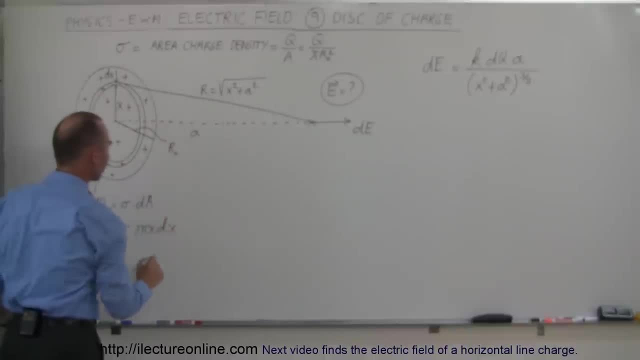 circumference times the thickness, which is DX. notice: I use the variable X for the radius of the disk so not to be confused by the, by the, by the full radius of the disk, and not to be confused by this distance right here. all right, so now we have the value for DQ, we can place that into our equation. 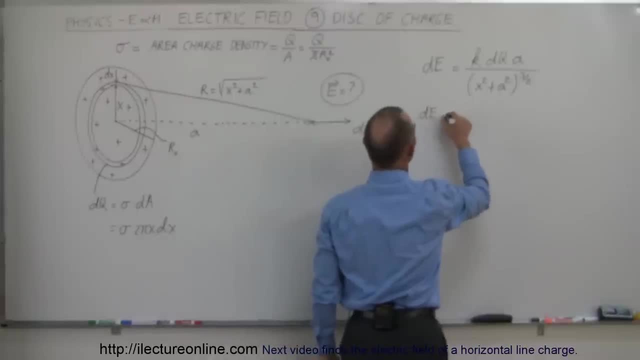 right there, so we can write that DE is equal to K times DQ and our DQ is Sigma times 2, pi, X times DX times a divided by x square plus a square to the 3 half power. all right now we should be ready to integrate, because now to find the total electric field. 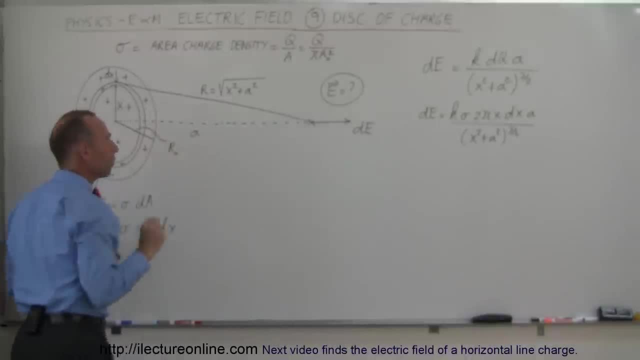 right here we're going to integrate across all the little ringlets. remember that the value for D is going to be horizontally outward because all the perpendicular components were eliminated by integrating around the whole little ringlet right here, so we only have to worry about the horizontal component DE. 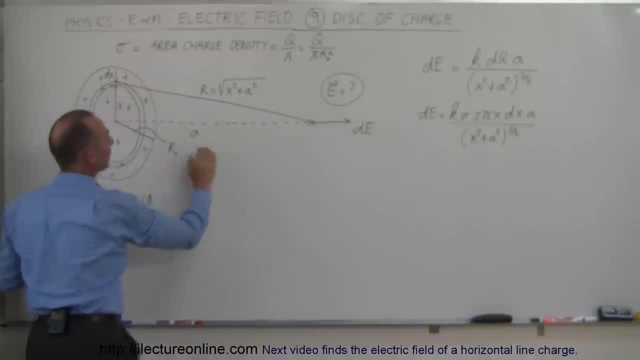 and then, if of course integrate across all the little ringlets, we'll get all the sums of DE's added together to get the total electric field. so the total electric field E is going to be the integral of all the little DE's, integrating from X equals 0 to X, equal the full radius of the disk. that means 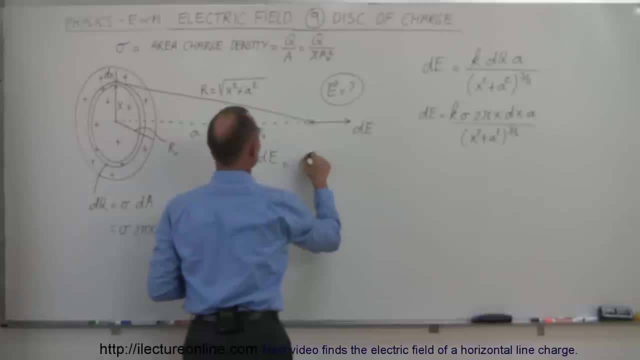 we're going to integrate this whole integral right there. so this is equal to the integral from X equals 0 to X equals the radius of the disk times K, Sigma, 2, pi, X, DX times a, all divided by X square plus a square to the 3 half. 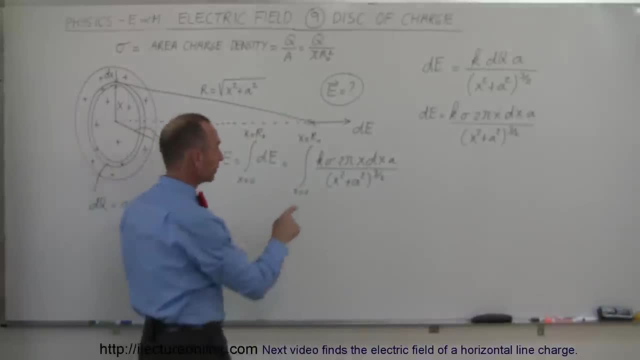 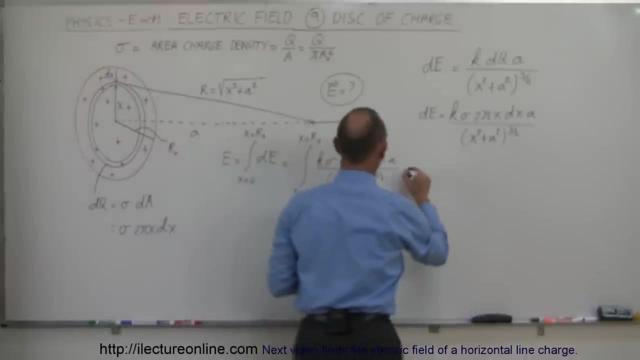 power. now, in this integral we have a lot of constants. notice that a is a constant, pi 2 Sigma K. they're all constant, they can all come out of the integral. so this is equal to K Sigma 2 pi a. and then we have left in the integral and let's 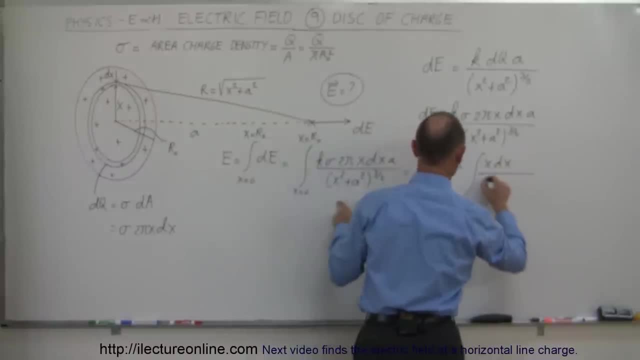 see here an X DX and in the denominator we have an X square plus a square to the 3 halves power from 0 to R, sub naught. so those, those are the limits of integration. now, this is a fairly straightforward integral because, notice, in the denominator we have an X square plus a square to some exponent in the 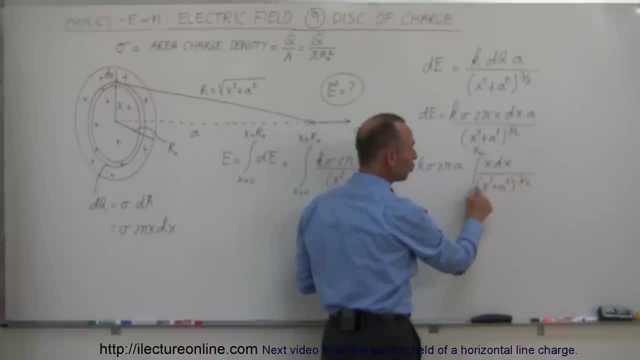 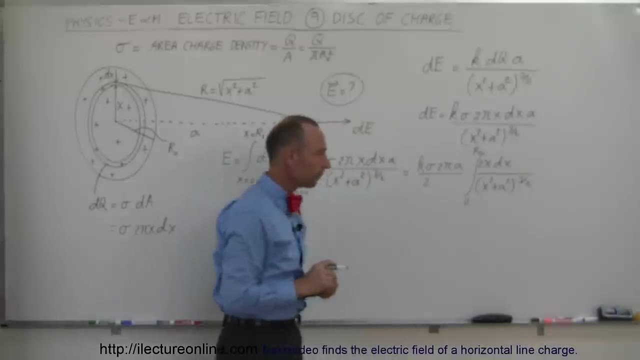 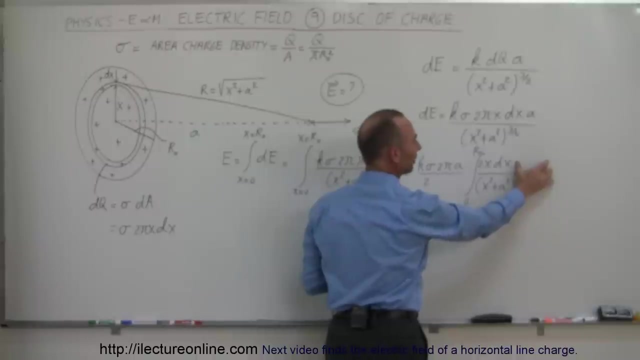 numerator. we have an X DX. the differential of the denominator is a 2x DX, so we need a 2 here. that means we need another 2 down here. now we can go ahead and integrate so this becomes X square plus a square to the minus 3 halves power when we bring it to the numerator. then when we 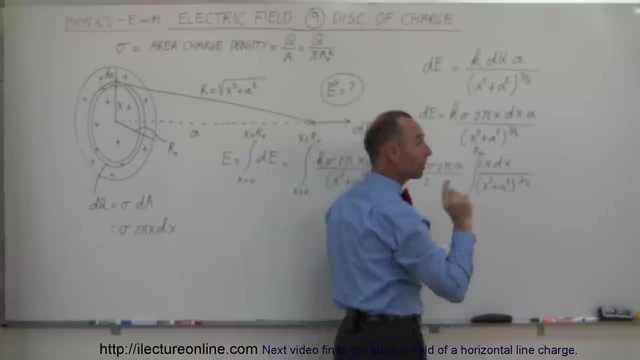 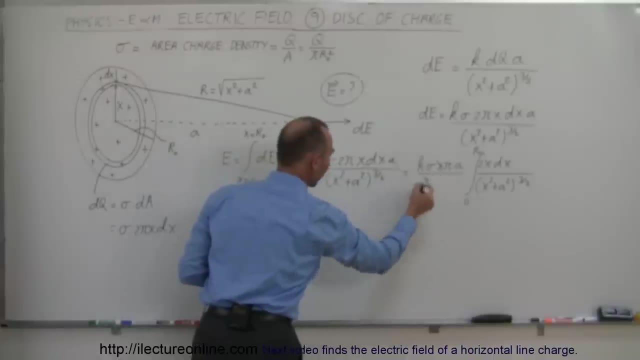 integrate, we add 1 to the exponent divided by the new exponent, then this is what we'll end up with then. so the electric field e is equal to all those constants, and notice that these twos cancel out right there. so I have K, Sigma, pi, a, and now we're going to integrate this, and so this now becomes 1 over. 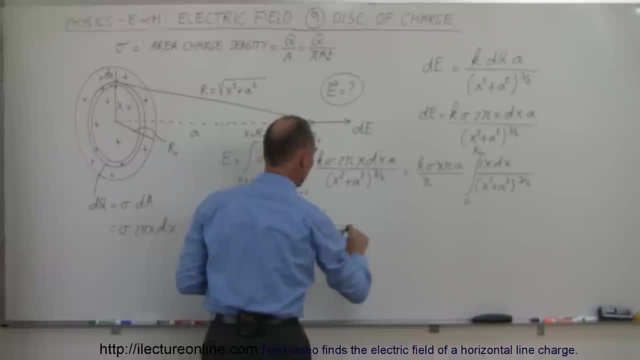 there. the first transpose is going to come down here into the mean square. it's going to get advantageous because there's the meaning of this formula, ucking it out and bring back the integral. and when we click in the numerator it's going to come out through this circle in here and we get. 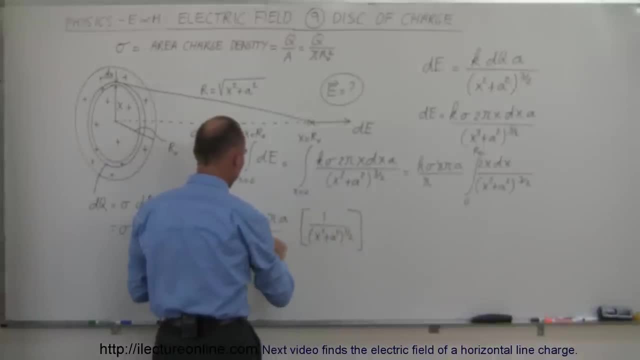 the hectangles, and here we have a Häring phenomena and that said, we generate these tough set elements. all right, now we've got the first воз complaint and this sense of Rico сос of s of v, and now that's it where we look into these industrial, true Biraz of burnt in the equation you. 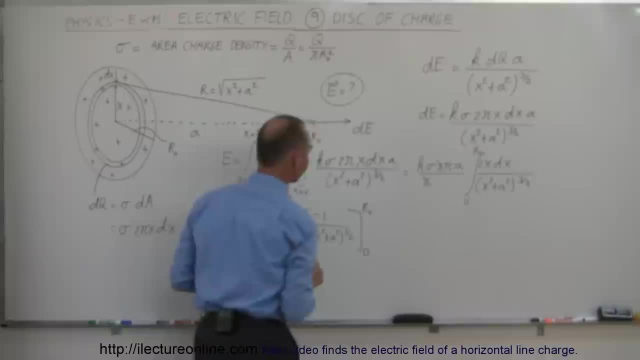 know, with a giora's line Yin Milan, such a thing as N Venant. okay, so the게요. All right. now we have to evaluate that when we plug in the upper limit, Let's see here, let's write it over there, so we still get k. 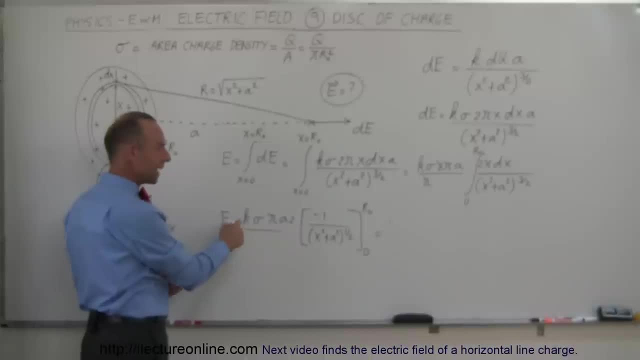 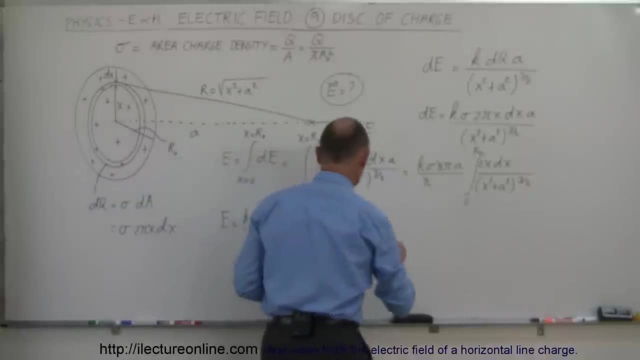 Oh, and by the way, to make this a little bit simpler here let's write k as 1 over 4 pi epsilon sub naught. That will simplify things a little bit. So we can write k as 1 over 4 pi epsilon sub naught. 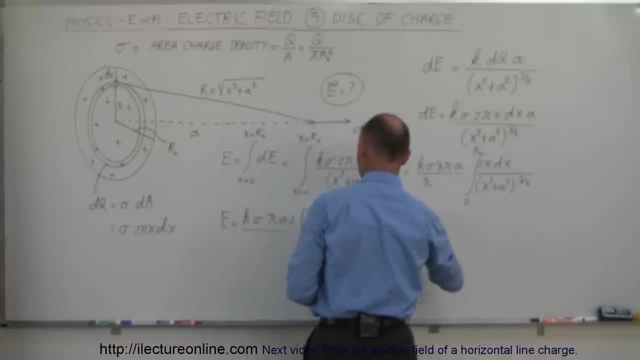 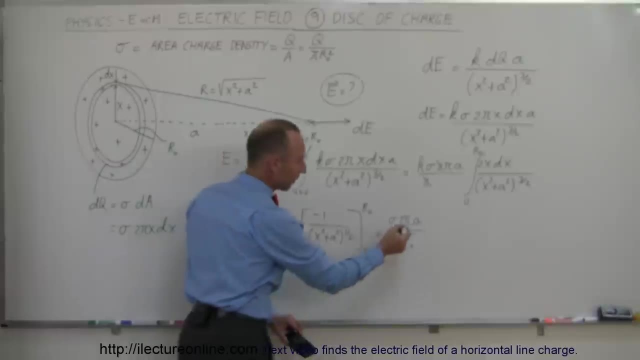 Then we're left in the numerator with a sigma 2 pi, and that will cancel out here and an a. So the reason I did that? because notice that the pi's cancel out and this 2 will cancel out with that. 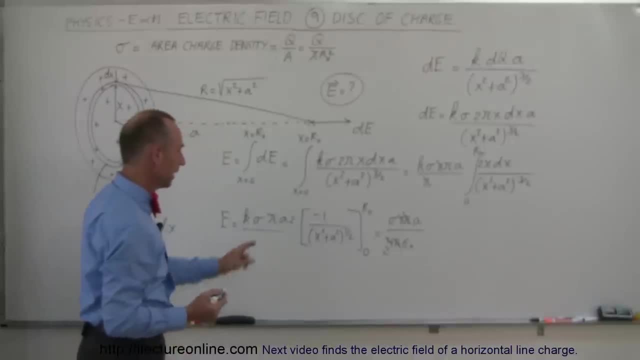 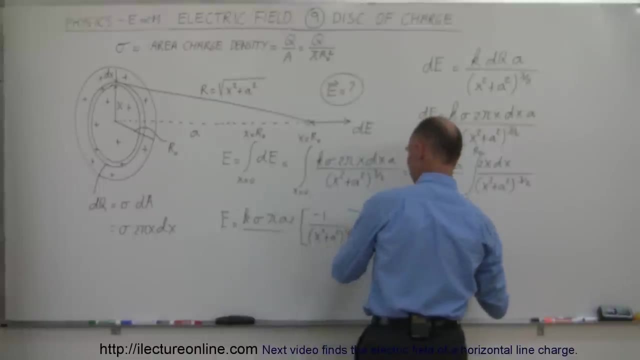 4 becomes a 2 epsilon sub naught in the denominator All right. and then when we evaluate this we end up with minus 1 over. plug in the r sub naught 4x. we get r sub naught squared plus a squared. 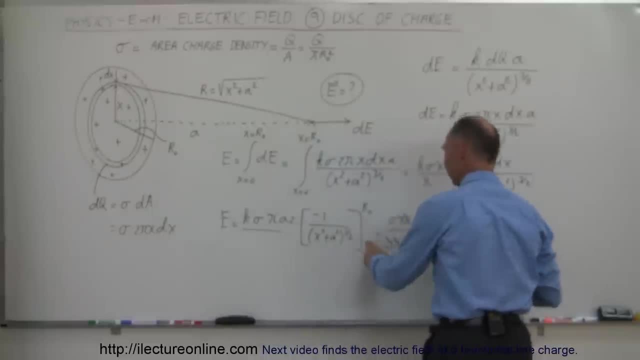 to the 1 half power and then minus when we plug in the lower limit. but since we already have a minus, there becomes plus 1 over. we put a 0 in for x, we get 8 squared to the 1 half power, or 1 over a. 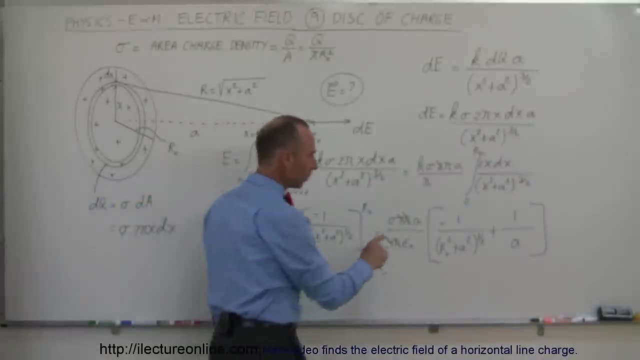 All right, almost done. Now notice, if I multiply this a in here, I'll get a minus a over this, and a over a gets me a 1, and I'm going to switch those around, because this is positive and this is negative. 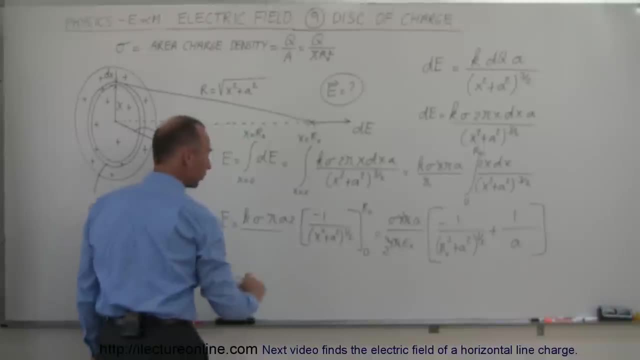 so then I finally can say that the electric field is equal to. I'm left in the numerator with a sigma in the denominator with 2 epsilon sub naught times. so a times 1 over a becomes simply 1 minus, because I still have the minus here. 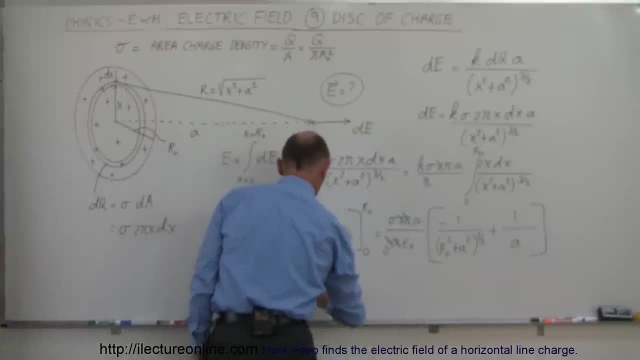 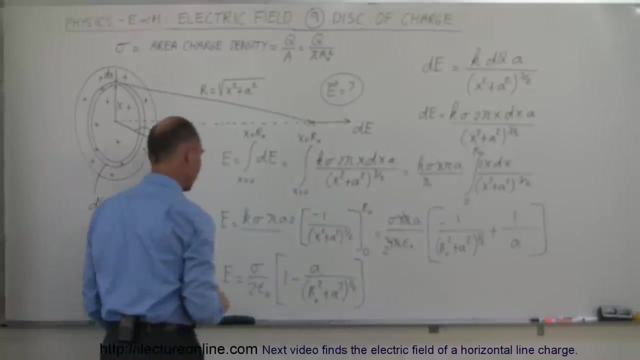 so that becomes a divided by the quantity r squared, r sub naught squared, plus a squared to the 1 half power. and now that gives us the electric field strength at this location due to this charge disk, If I want to make it into a vector. 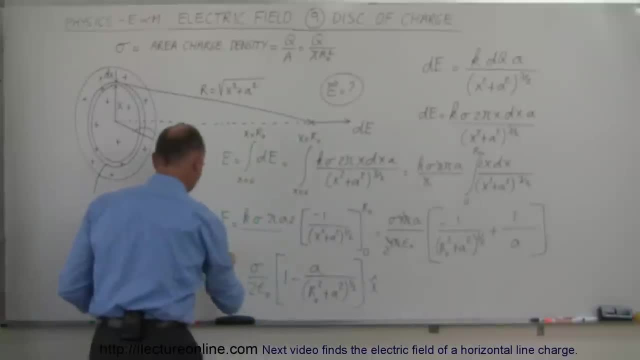 I put a vector symbol here and put the unit vector in the x direction there, and that will then be the electric field to the charge disk. I know that algebraically we can still write this in different forms, but that is one of the more simple forms to leave it as.